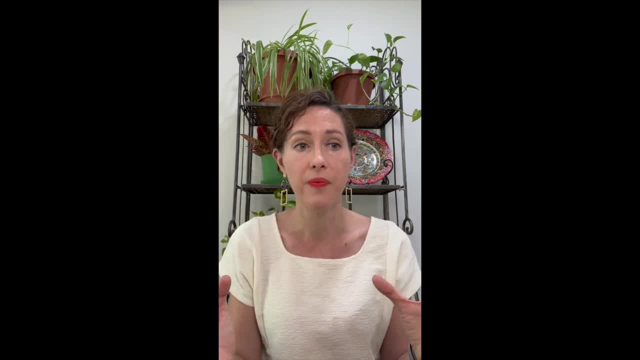 know it is not a ban. It is not a ban. CERCLA regulates cleanup of chemicals, So it's really the law that comes into play once a chemical has been released into the environment. People have been exposed to the environment. People have been exposed to the environment. People have been 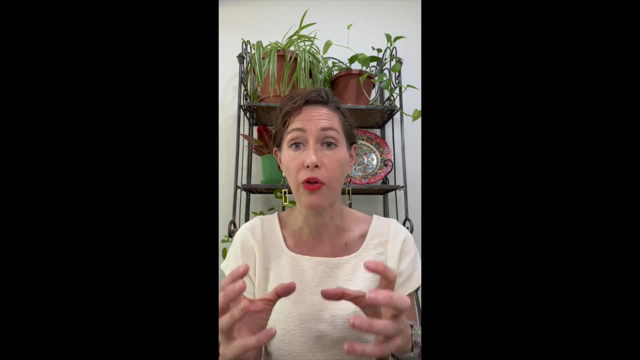 exposed to the environment, But it doesn't regulate the use of that chemical. There are other environmental laws, like the Clean Air Act and the Clean Water Act and the Toxic Substances Control Act, that are focused on the ongoing uses of a particular chemical, but not CERCLA. 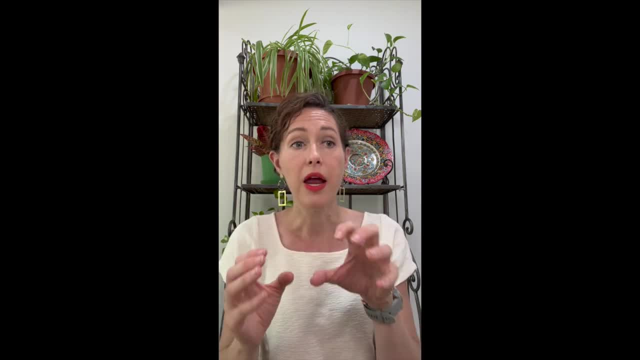 CERCLA is a cleanup statute, And so instead, what CERCLA does is it governs the cleanup of sites contaminated by the release of these hazardous substances, And then it allows the EPA to recover costs from the polluters that are responsible for that pollution. And so 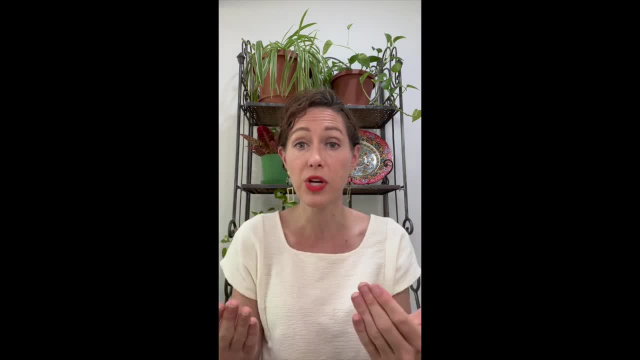 it allows the EPA to clean up And it also, if EPA is expending resources and some taxpayer money to do that cleanup, then EPA can take back some of those costs. And over the more than 40 year history of Superfund, designating a chemical as a hazardous substance has actually rarely led 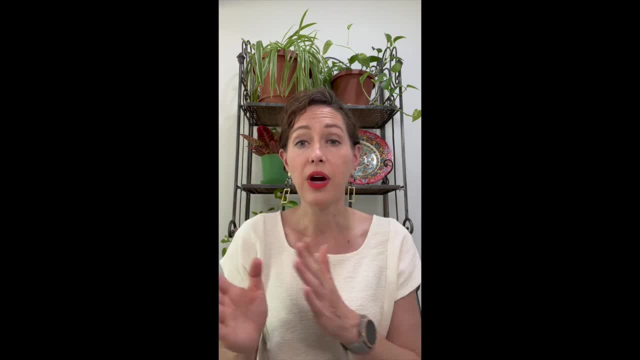 to manufacturers stopping to use it. In fact, CERCLA hazardous substances are used by manufacturers every day and often in large quantities. So right now there are roughly 800 different substances on the CERCLA hazardous substance list or the Superfund hazardous substance list, and almost 700 of those chemicals have 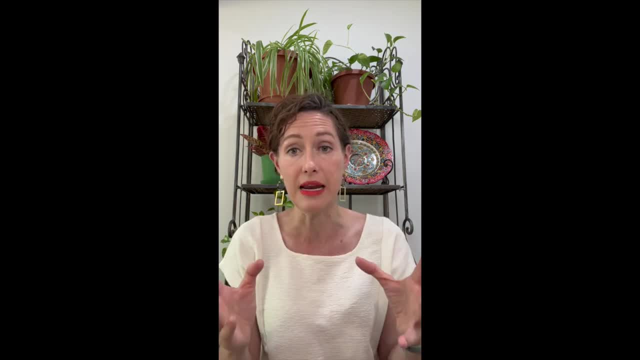 been on that list for more than 40 years, since 1980, when the law first passed, And EWG did an analysis in 2019, a couple of years ago- and we found that at least three-quarters- around 600- of those chemicals are still in active use, most likely. 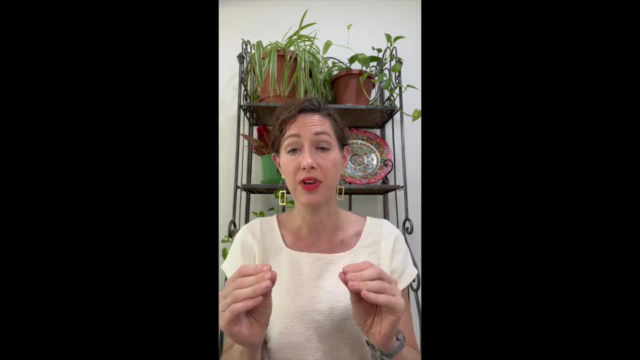 And, moreover, nearly half of those CERCLA hazardous substances, or 339 of them, were not only still in use but were likely produced in large quantities. In fact, sulfuric acid is a good example: This is one of the most produced. 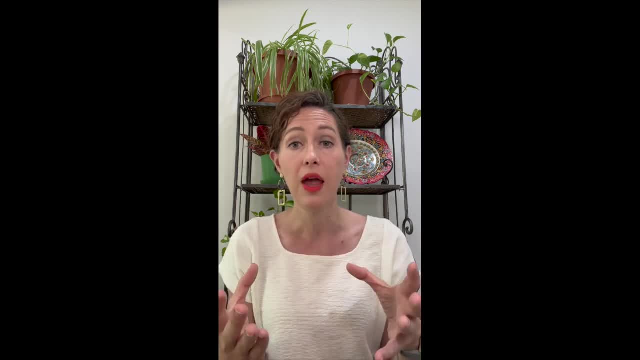 and most widely used chemicals in the world, and it was on that original list. It has been a CERCLA hazardous substance for more than 40 years, but manufacturers have found a way to continue using it. continue using it in large quantities without releasing. 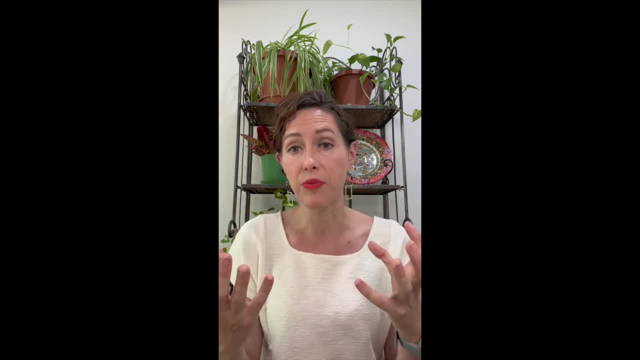 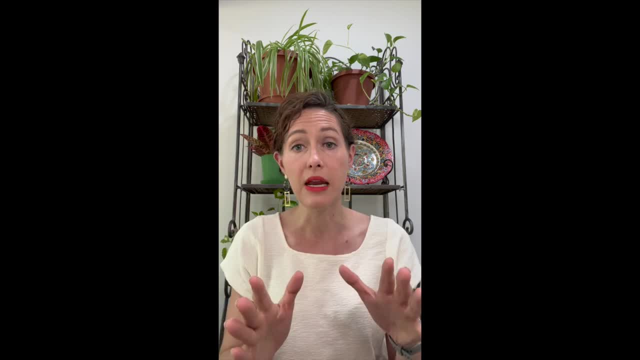 They have been recycling industry products. They have been recycling industry products. They have been recycling industry products And they have falsely claimed that, designating PFOA and PFOS or any other PFAS chemical as a hazardous substance, that it would ground airplanes. 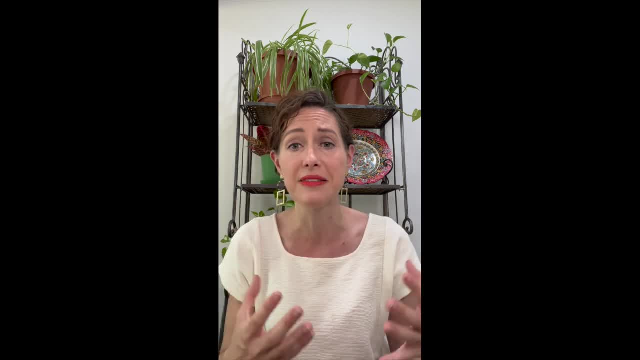 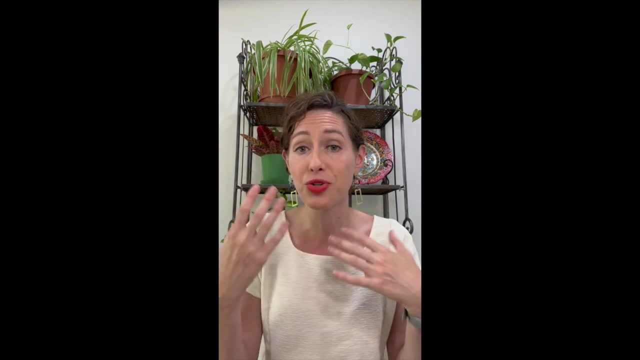 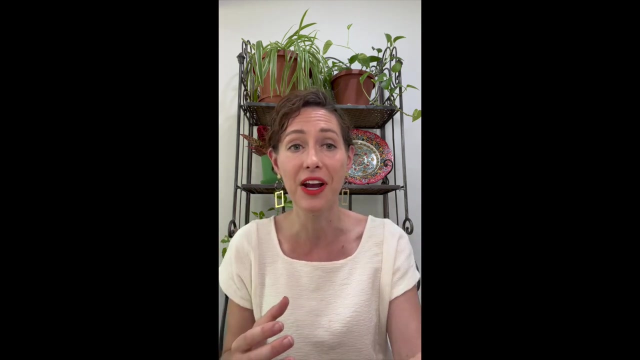 It would end the use of life-saving heart stents and infants and other people, and it would require us to throw off our personal protective equipment, the surgical masks that we have all been wearing for the last two years. So, for example, in one hearing a legislator 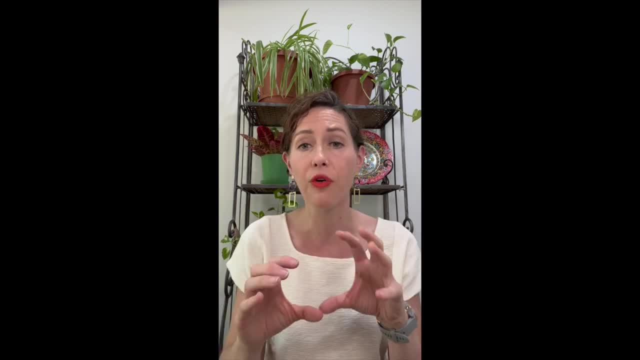 warned that labeling all PFAS as hazardous would provide a direct threat to FDA-approved drugs and devices, because PFAS is used in some of those drugs and devices which could lead to lives lost. At the same hearing, another legislator said that designating PFAS as a hazardous substance was 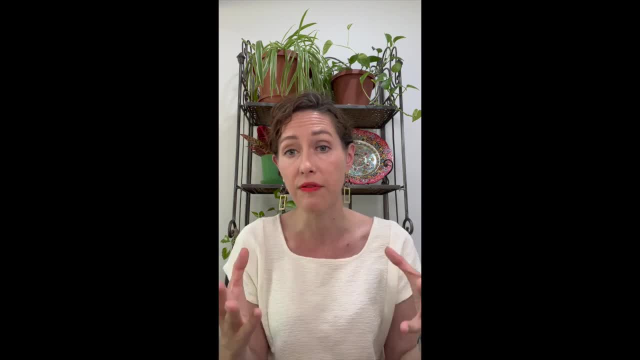 proposing to end the use of masks because many of them contain PFAS, And I just want to say that this is nonsense. It's simply not true. Just as circular hazardous substances continue to be used by many industries even after they are designated, a lot of circular hazardous substances are also. 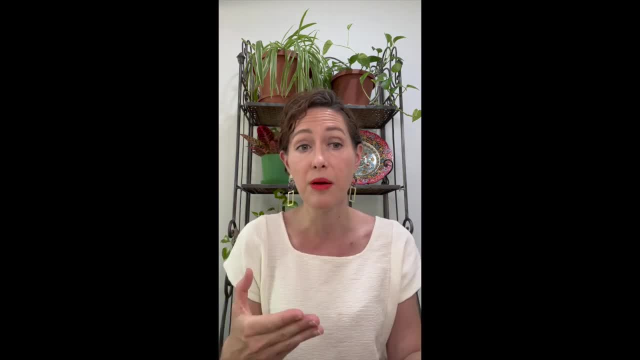 used in the medical field. Ethylene oxide is one example. It's used to sterilize medical equipment. A couple of other examples: xylene, toluene and formaldehyde- are all used to preserve tissue specimens. Mercury can be used in dental amalgam. 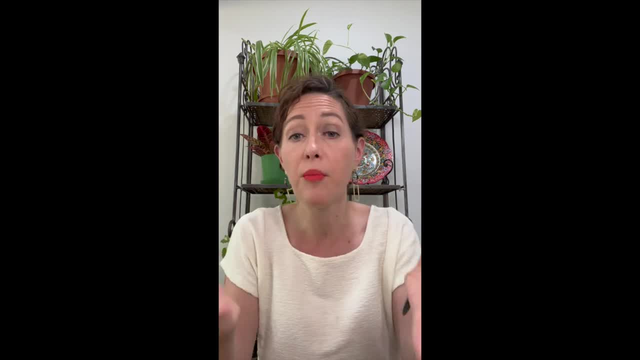 products, And so, as I said, this is nonsense. It's simply not true. Just as circular, hazardous substances are used to preserve tissue specimens, And so, as I said, this is nonsense. It's simply not true. And so, as I said, this is nonsense. It's simply not true. And so, as I said, this is just a number. 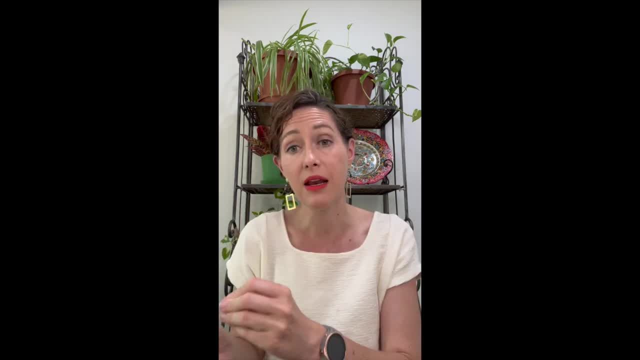 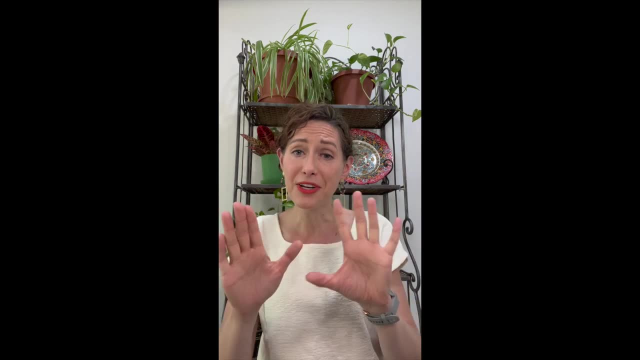 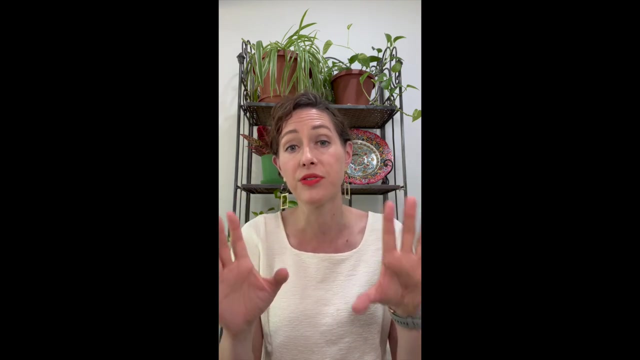 of examples where hazardous substances have been designated, but it has not created a de facto ban on the use. But here's actually the most important reason that designating PFOA and PFAS again, those two most notorious PFAS, forever chemicals. here's the most important reason. 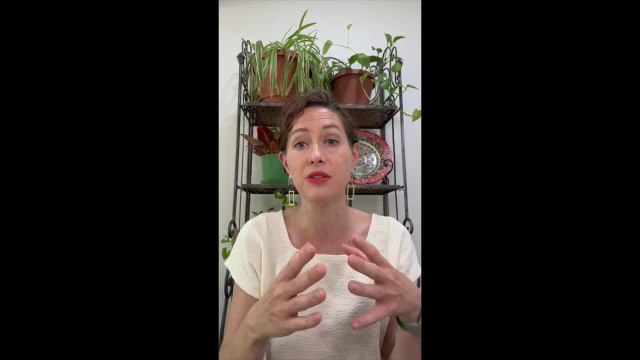 why designating those PFAS as hazardous substances would not be a ban. PFOA and PFAS have already largely been abandoned by industry because of a 2006 stewardship agreement that the major manufacturers of those chemicals signed with the EPA, And so you can't create a. 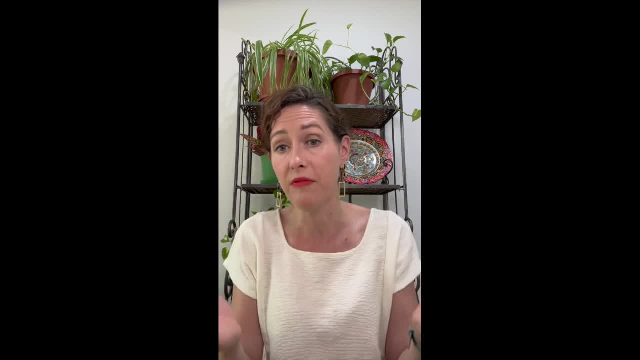 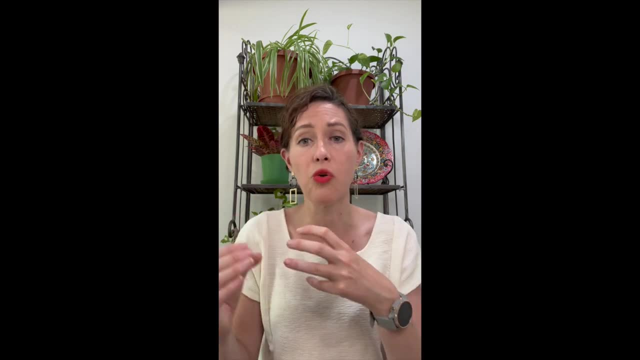 de facto ban of chemicals that have already been phased out, And so this is just another example of how saying that this is going to create a ban, that it's going to get rid of medical devices and pharmaceuticals that people rely on, It's just not true. It's simple. 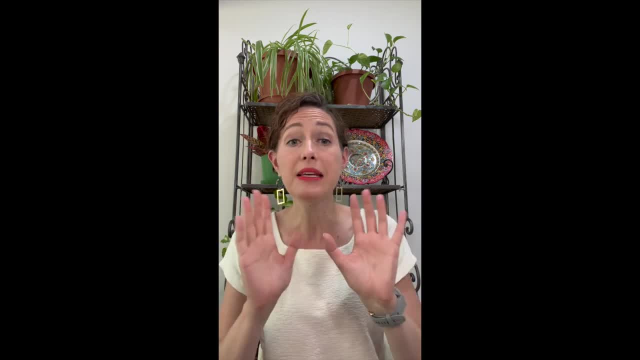 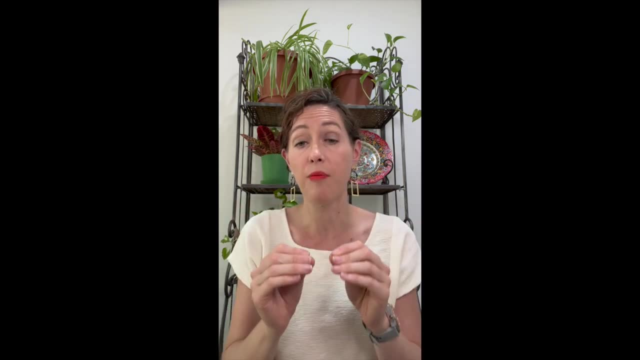 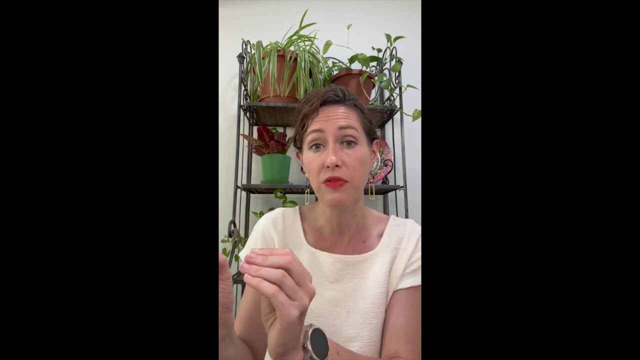 It's simply not true, But here's what EPA is proposing to do and why that's important. So the Superfund law distinguishes between chemicals that have been designated as hazardous substances, as the EPA is proposing to do for PFOA and PFAS, those two PFAS chemicals. 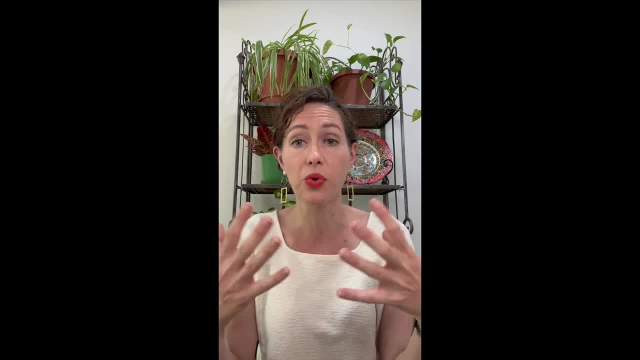 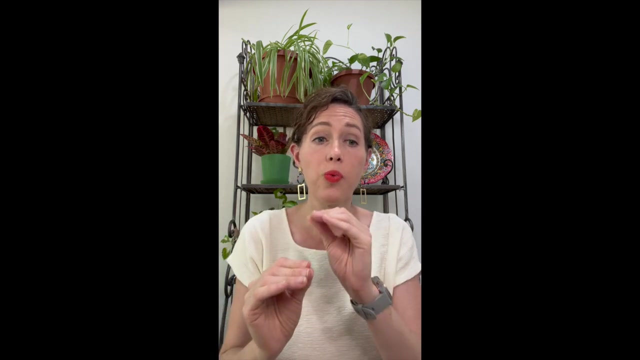 and chemicals that are just considered pollutants or contaminants, And so under the current law prior to the EPA announcement, PFAS chemicals are considered pollutants or contaminants but not hazardous substance, And that difference it really limits the power of the EPA and states and communities to clean up PFAS pollution. So the first difference is by making something a hazardous substance designation, you create a reporting requirement for any time you release that substance over a certain threshold. And when you release over that certain threshold you report. it triggers an investigation. Regulators will look into that release. 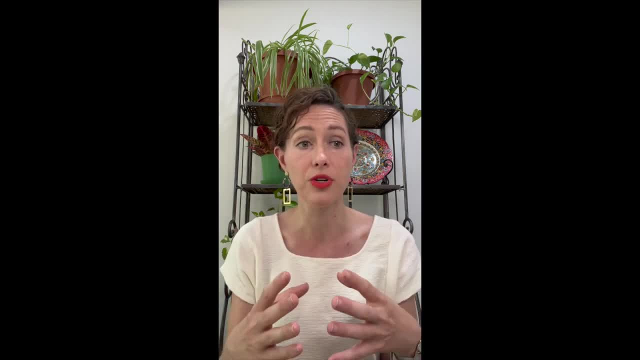 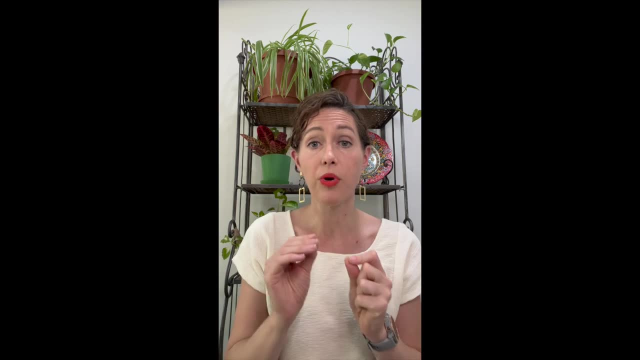 into the air, land or water that's exceeding that threshold and determine whether or not there needs to be a cleanup. By contrast, when something is just a pollutant or a contaminant, you have to show that there is an eminent and substantial danger. 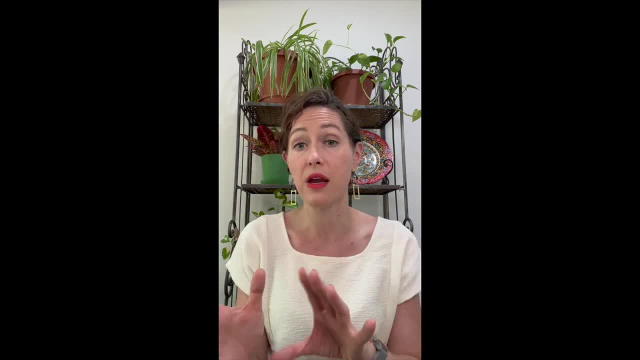 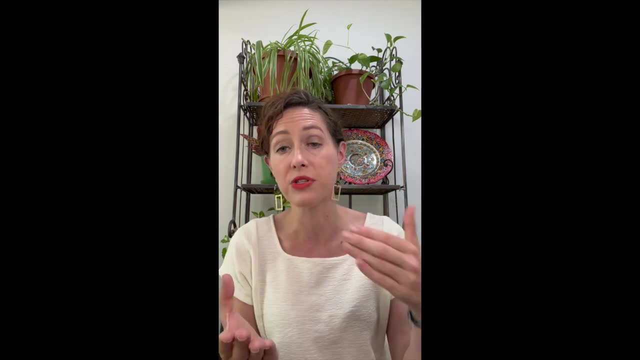 that's the legal test to public health before the site can be investigated and cleaned up, And so that is, just from a legal perspective, a much higher bar to meet then simply being able to show that you have released them out over the threshold that has been established. 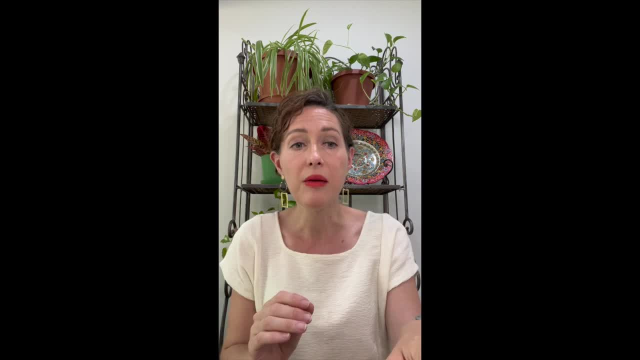 for reporting. And then second, even when the EPA can meet that high bar, that eminent and substantial danger, the EPA's actions that they can take in response to that are much more limited. And perhaps most significantly is the EPA's ability to. 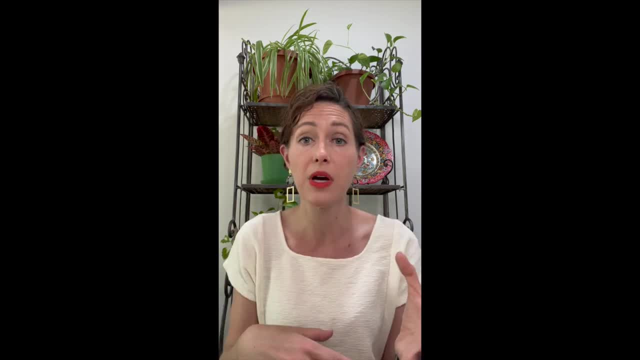 use its own funding to initiate a cleanup. Sometimes you have a site and it's not easy to immediately identify who the responsible parties or polluters are, or there's just a really urgent need to clean up, And so in that case, what the EPA may do is take some money. 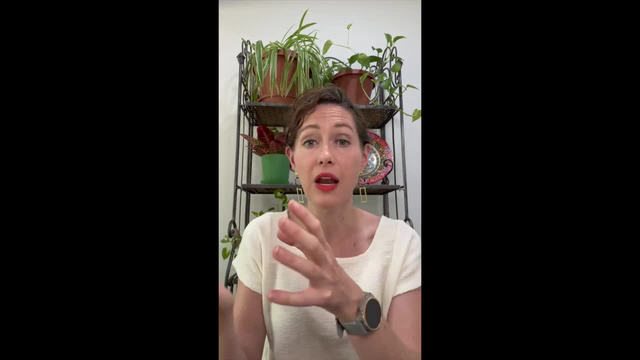 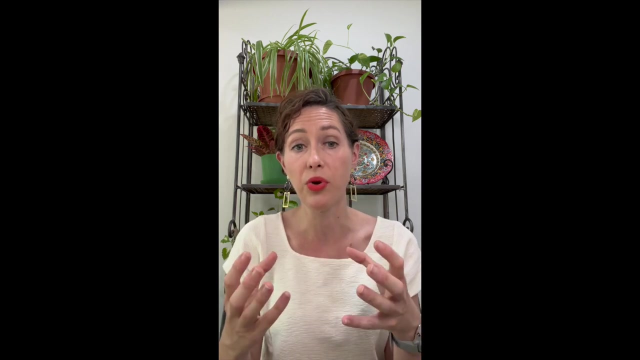 from the Superfund, as it's called, and initiate that cleanup And then EPA can identify the polluters, the responsible parties, and sue them to recover some of their costs. But you can only do that if something is a hazardous substance. You can't do it with just a pollutant or 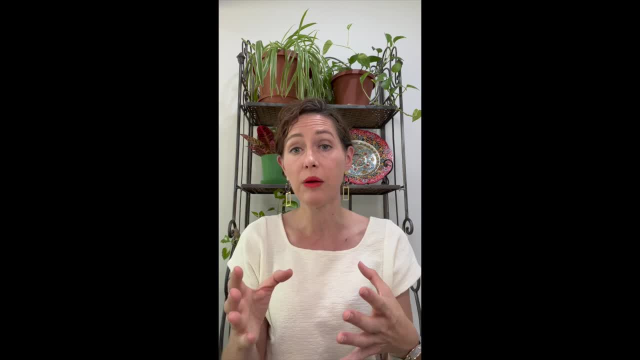 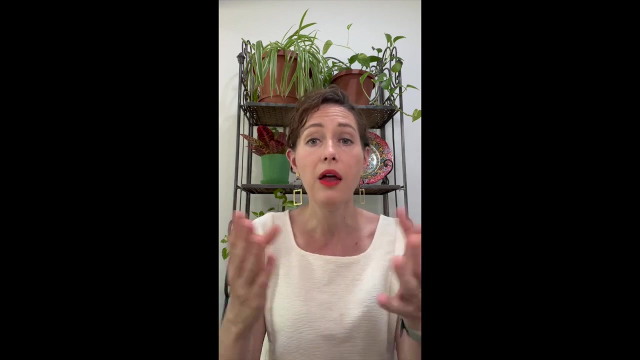 contaminant. And then third, practically speaking, because the Superfund program has limited resources, as do many EPA programs, it tends to prioritize hazardous substances, in part because it has those additional mechanisms and things that they can do. Another difference: EPA can order a cleanup. 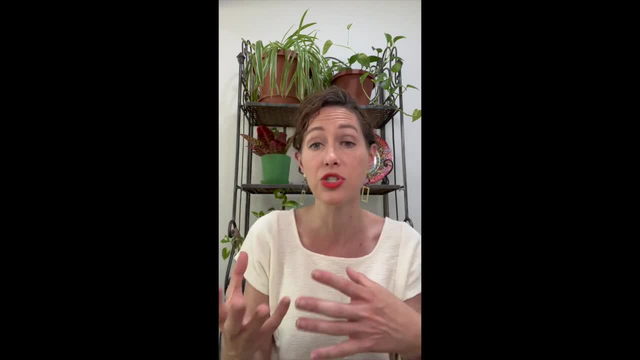 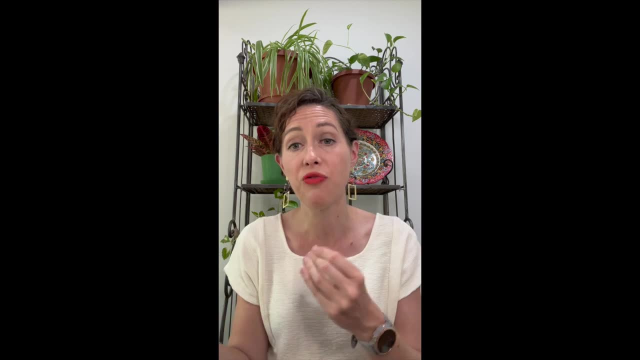 for a hazardous substance, which they can't do for something that's just a pollutant or contaminant, And so you can't do that with just a pollutant or contaminant. Giving EPA more power will also allow them to shift more resources to address forever chemicals. 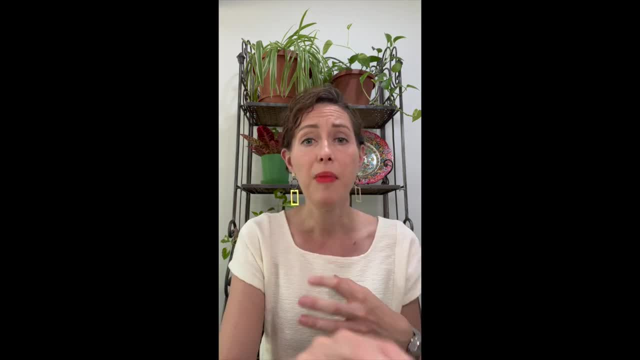 at existing and at new Superfund sites. And then, finally, the Department of Defense is a major PFAS polluter because for more than 50 years it used a special kind of firefighting foam that was laden with PFAS and then would release a lot of that foam, And that foam got into the ground and 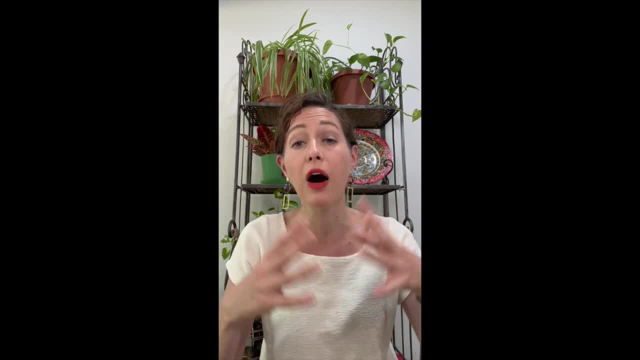 got into the drinking water and contaminated hundreds of communities. But despite this direct connection to PFAS contamination, the Department of Defense has really been dragging its feet in cleaning up those contaminated sites, And so the section of the Superfund law that focuses on federal actors like the Department of Defense is largely focused on hazardous substances And so creating this hazardous substance. 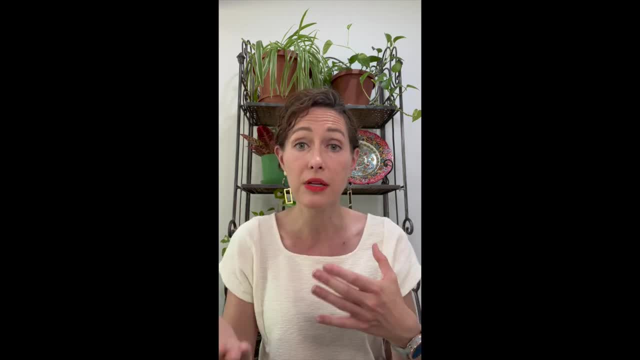 designation will then make it easier for those communities that have been polluted by the Department of Defense to hold the DOD accountable and for the EPA to hold the DOD accountable because of their role in polluting so many communities. And so, just to summarize: is hazardous substance designation a ban?